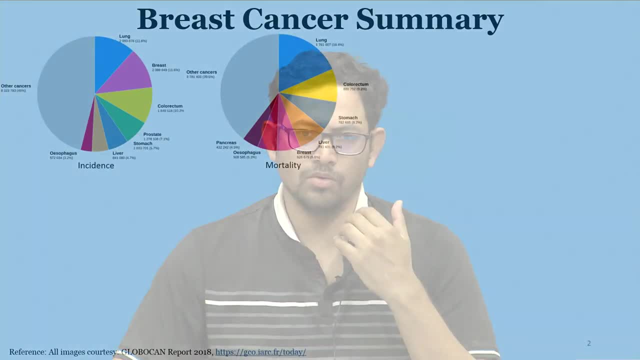 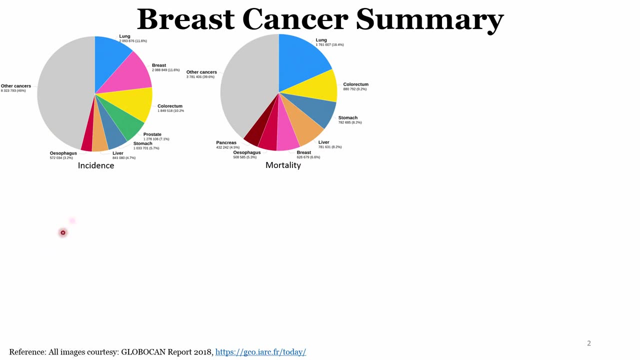 So, first thing is the: why breast cancer? ok, So the? so let me just switch on the laser pointer. yeah, So, as you can see, breast cancer is the cell number second most highest number of cases. where you see the incidence rate and in the 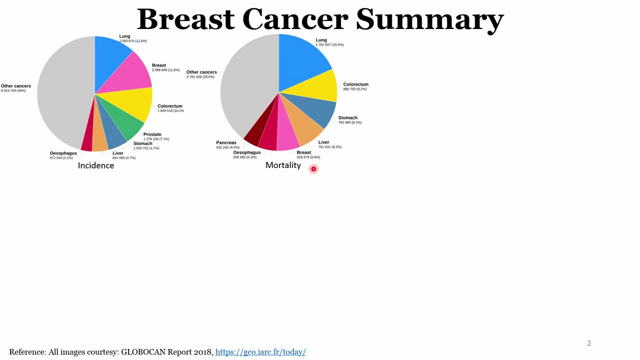 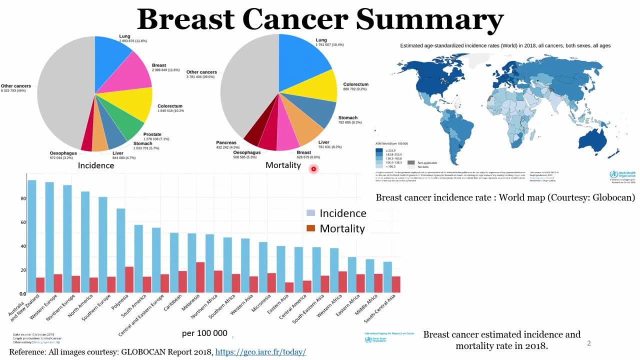 case of mortality is the number fifth number of cases where you see the breast cancer over here. Now, once you try to see what is the incidence and mortality rates throughout the world. Now what I try to do is what try to show over here is the profile of the different 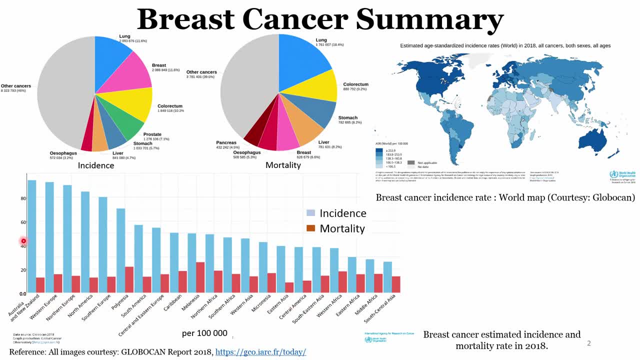 different countries- ok, countries on the x axis and the y axis. we have plotted the incident rates in the blue graph and the red graph is for the mortality. What do we see over here? We see that for developing countries such as Australia, New Zealand, Europe and America, you can see that 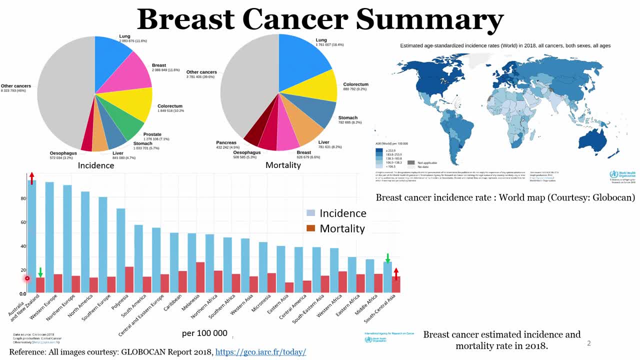 there are large number of incident rates as compared to the mortality. So mortality is fairly less as compared to the number of incident rates. but if you see less developed countries or developing countries such as India, South Africa, what you see is the incident rates. 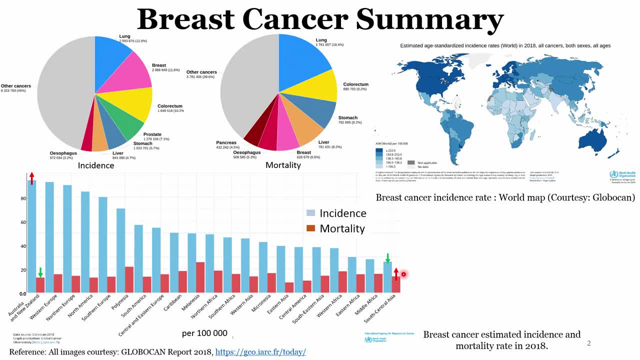 are lower, but the mortality rates is comparatively higher than the developed countries over here. So why is this kind of a question that is arriving over here, that why the incident rates, which is lesser, but then also the mortality rate, is lower. So why the interest is comparatively, or its more as compared to developed countries? 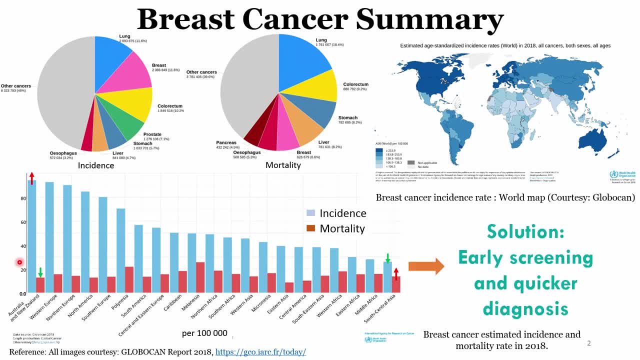 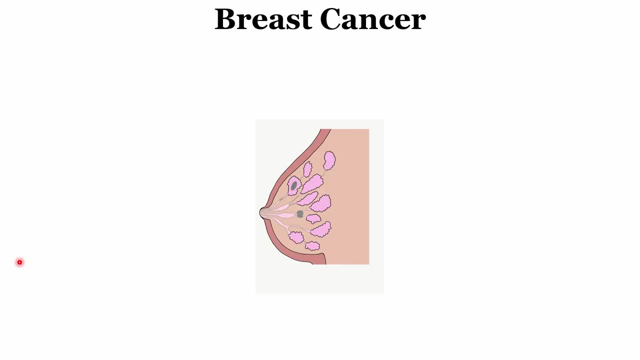 The answer to this question is about the early screening and quicker diagnosis for breast cancer disease. So we are going to talk about how you can approach this breast cancer disease. how do you diagnose the breast cancer using the optical techniques? Before approaching the breast cancer with the optical techniques, we should always know about the basics of 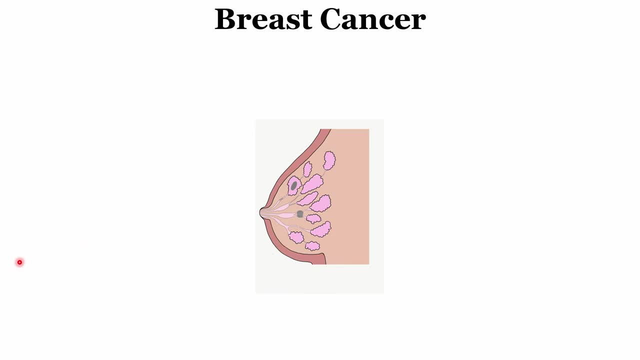 the breast cancer and what are the different kinds of cancers that you can diagnose with the techniques that we have over here. So this is how the anatomy of the breast looks like. what we have is the lobes over here. we the lobes is where the milk is created and then it is supplied through the ducts. 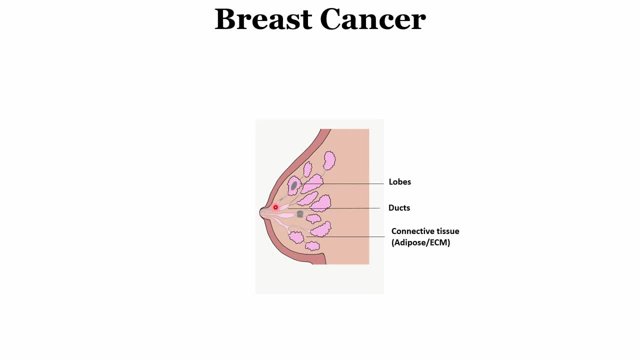 to the nipple And the other brown colored structures are the connecting tissues, that is, the adipose and the extracellular matrix. Now you can see the structures, such as the grey structures that you see over here. it is seen in the lobes, within the ducts, as well as when it 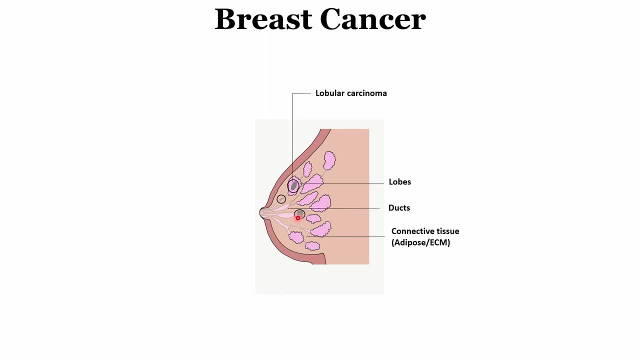 is spreading out from the ducts, The first thing that you see is the disease which is generated within the lobes and that is known as lobular carcinoma. and if I just zoom into the duct part over here and you can see over here, the grey part, over here, the grey region which is surrounding 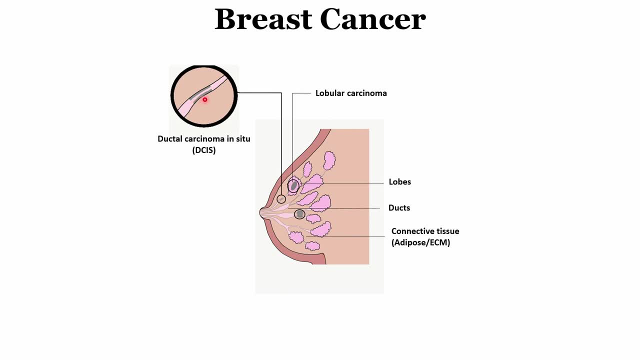 to the inner surface of the ducts, and this is in situ, that is, it is still within the ducts. it is not start to spread yet, and this is known as ductal carcinoma in situ, is also known as DCIS. in short, Once it starts to invade or come out of this, 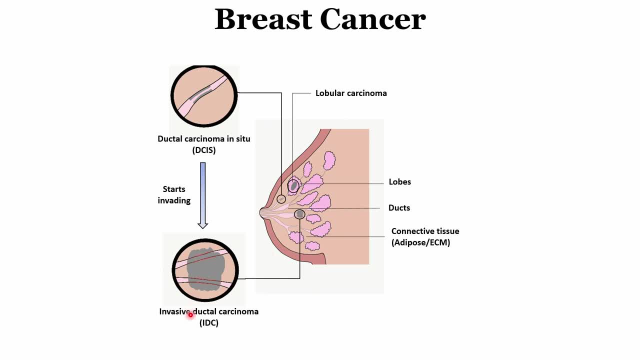 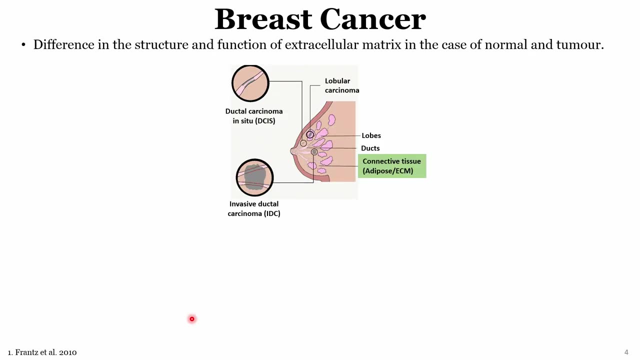 ducts, then it is known as invasive ductal carcinoma and around 80 percent of cases you see such kind of invasive ductal carcinoma when the breast cancer is diagnosed. So let us go forward. So the first thing that comes in the mind of the clinician or 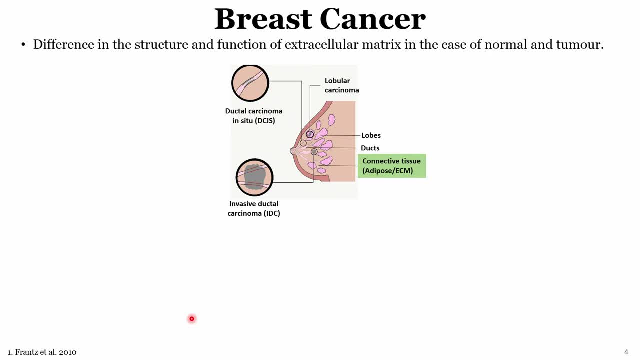 the engineering person who is trying to develop a breast cancer diagnostic tool is that: how do we differentiate this different types of cancer? Before do that you should also understand, or one should also understand, what is the constituents within each of these components of the breast cancer, or a constituents of the breast cancer. 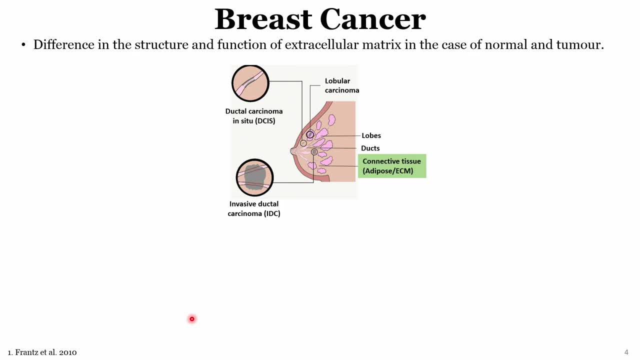 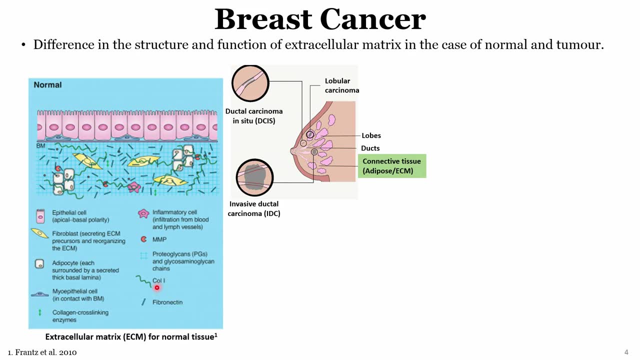 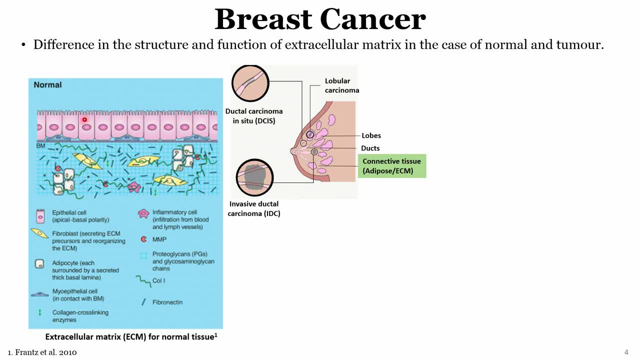 the left side. In the case of normal tissue. what you observe is this: epithelial cells or this basal cell membrane are like very isotropic, that is, all are arranged in a very uniform manner over here. As you can see, over here they are kind of. 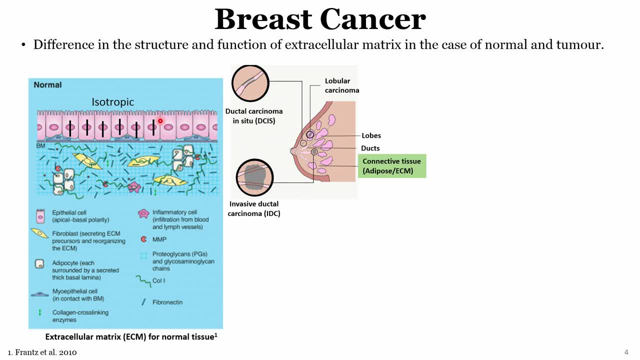 pulled to a certain direction over here, and that is the case when it is normal. You see all the other collagen fibers, you see the adipose tissues, the fibroblast. all of them are placed inside this basal membrane that is inside over here, and that is the grey part. 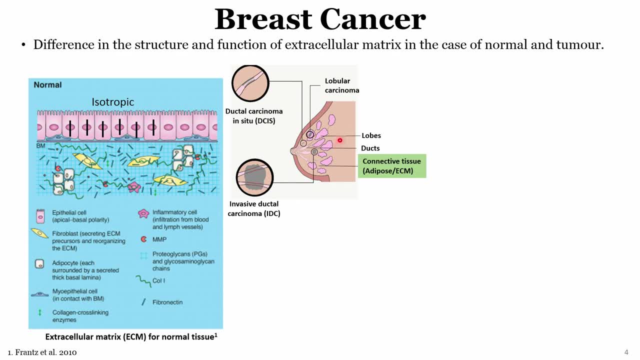 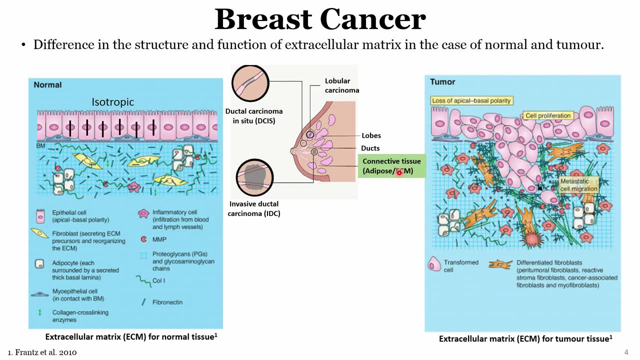 that you see, or not the grey but the brown color that you see over here. But in the case of the cancerous tissue, what you see is it is not isotropic anymore. what you see is anisotropic arrangement of the cancerous basal membrane cells over here. ok, 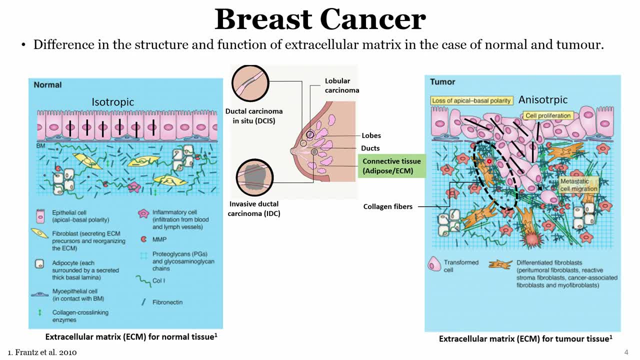 And you can also see this collection of the collagen tissues which are surrounding this basal membrane, tissues which are trying to go inside, Now the extracellular matrix. So this is the main difference between the normal and cancerous tissue or a tumorous tissue. Tumour tissue is basically which has still not spread. 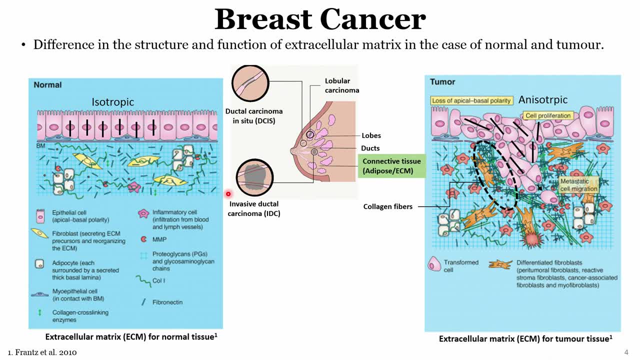 through the other parts of the breast and through the body, through the lymph nodes, and it is basically very anisotropic. It is kind of arranged in a very random and unorganized manner. Ok, looks good, So let us go next to understand the ducts. The ducts: when you try to see the 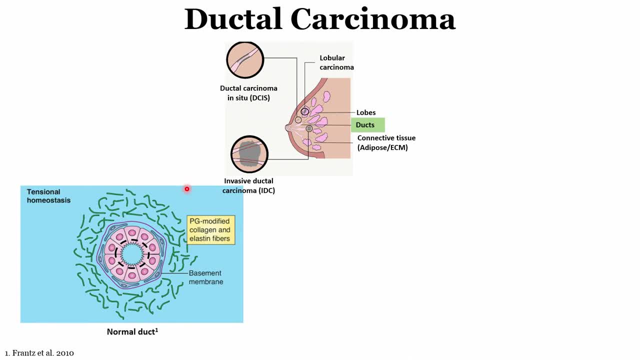 anatomy of the ducts, you will get a stress sketch, something like this. So it is a kind of a circular cylindrical structure where you see the basal cell membrane over here which is surrounding the ducts over here and through the center, the milk which is surrounding. 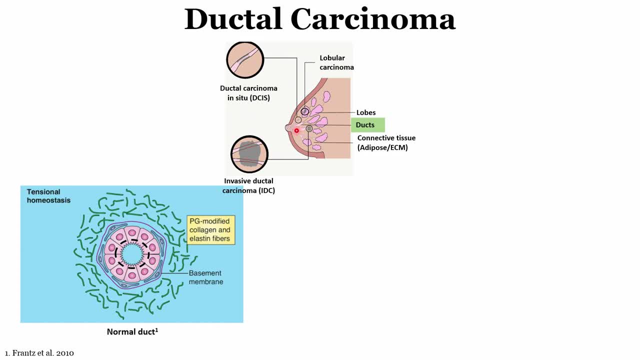 So this material is generated by this or created by this lobes is transported to the navel. ok, So this is the case when we are talk about 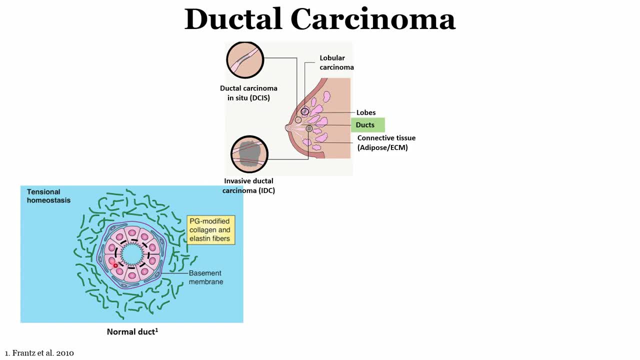 the normal duct profile. ok, It is nicely arranged in a circular manner. The stress being developed from the internal and outer is like equal, So it maintains it's circular shape and the other part is As you. 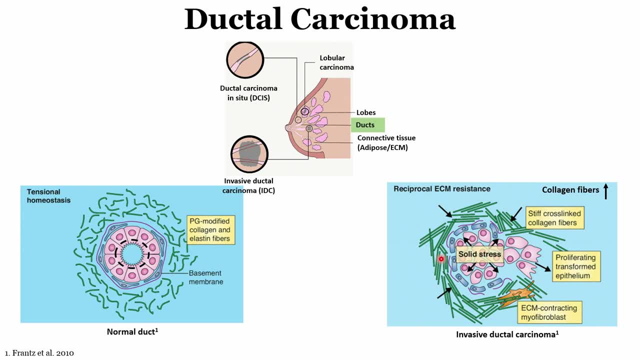 see on the right side, what you see is a case when the duct is undergoing a transformation towards the tumor. So what you see over here again is the random nature or random arrangement of the ducts over here. no milk can actually pass through this duct over here because there 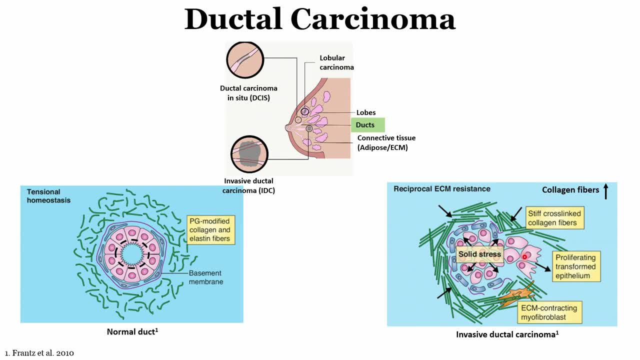 is no more hollow space in the center. You can also see that this basal cell membrane is now coming out of the collagen fibers that were nicely keeping surrounded by this around this duct profile. but now it is kind of broken and the cells which are, which are now undergoing 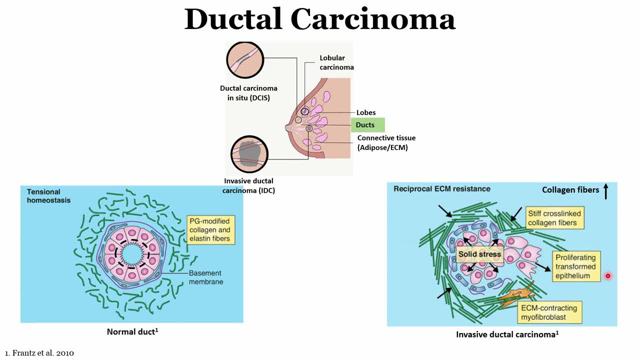 this cancer metastasis. It is now spreading to the other parts of the breast. ok, So this is what you see. is this the now the stress is not equal- which is now coming out towards our muscle here. So this is not averse to the pressure, so this is not averse to the 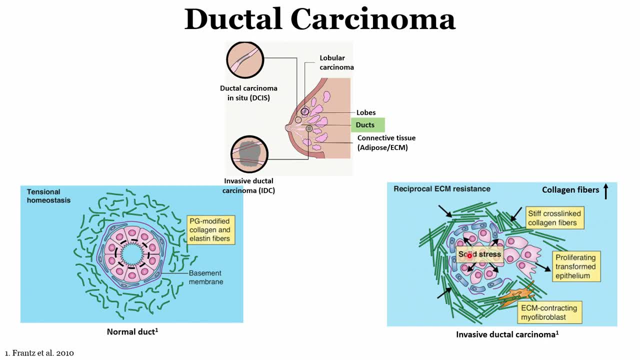 pressure. So this is what this is. So this is the pressure. So this is the pressure outwards as well as the inwards, So it is now unequal. there is a change in the equilibrium balance over here, and what you observe is that the solid stress is trying to pull outwards. 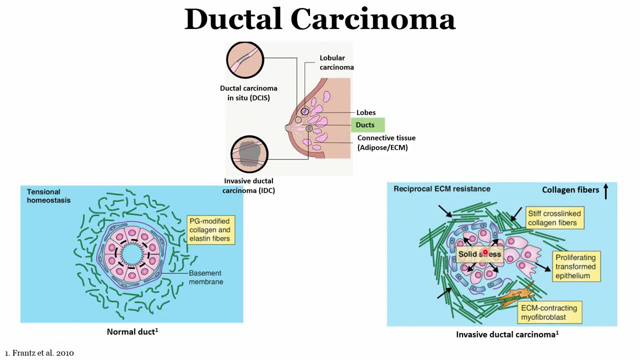 and, at the same time, the stress, which is acting like a resistance by the extracellular matrix, is now pointed inwards. In addition to it, what else you can see is that there is large number of collagen fibers that are now being present in this structure over here, and this is going to be one of the main factor that we are going to take at a 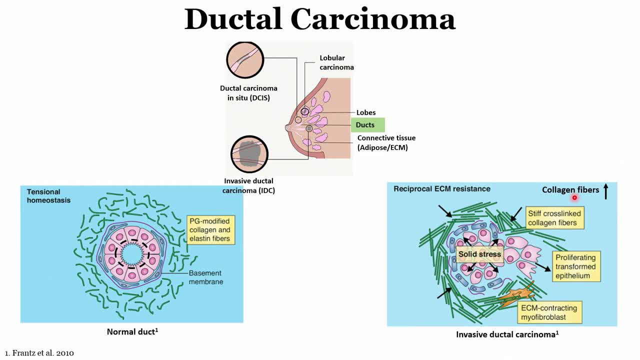 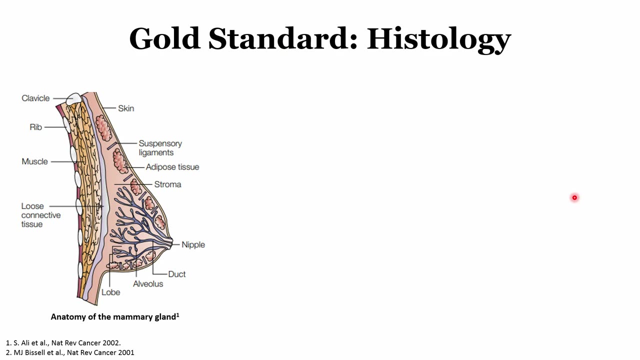 later stage which changes the properties of these biological tissues, such as the density of the tissue, which eventually changes the optical properties of the tissues, such as the scattering coefficient. So when we talk about How do we diagnose the breast cancer, There are different techniques and the one technique 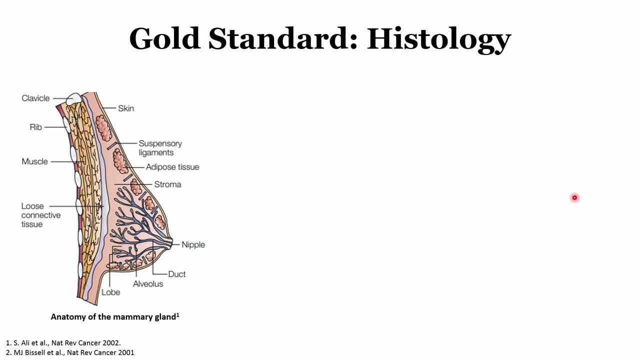 which is used worldwide, is known as gold standard. The current gold standard to diagnose breast cancer, the type of the breast cancer that is, the pathology of the breast cancer, is to use the histopathology where you have the H and E test, hematology and eosin stain. So 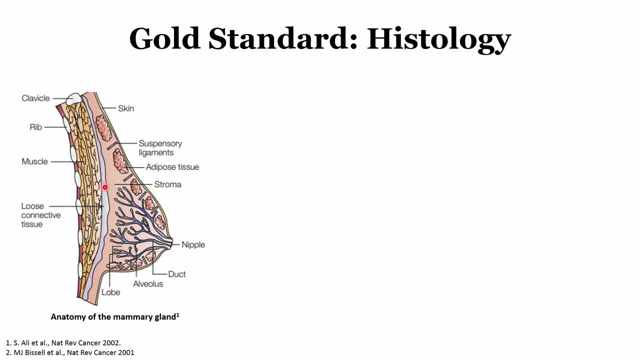 what do we do is So this: on the left, you see the breast in the case of a normal breast, and what you do is you take a small part of this breast using the biopsy gun or the biopsy punch or biopsy needle. You cut it into a slice of hundreds of micrometers thin slice of tissue and then 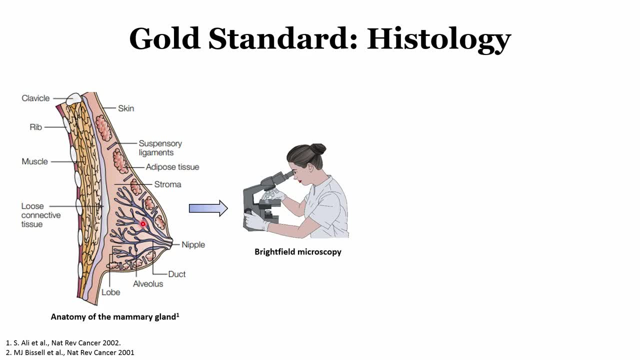 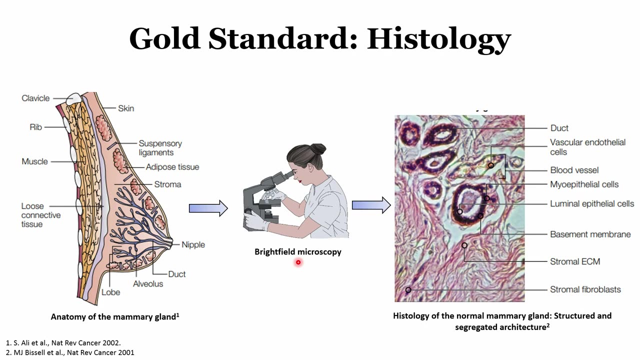 you stain that tissue and then put it under the slide with the cover, slip on top of the top of it and see it using a bright fill microscopy technique. ok, So this technique is used to understand the pathology of the breast cancer, and this is on the right side, what you see. 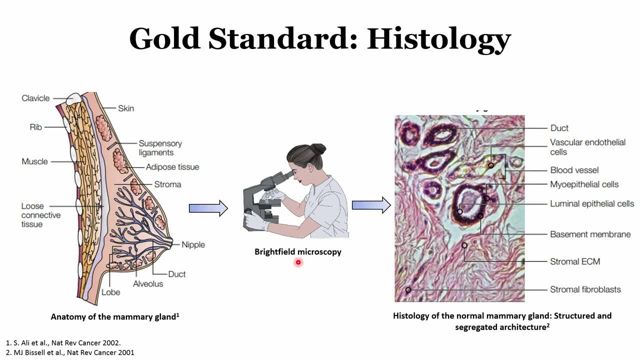 is a normal breast cancer histopathological test. So you can see nicely the ducts which are being formed over here. it is nicely circular over here. you can also see the blood vessels over here. So this is the dark region over here where the blood is flowing over here. you can also 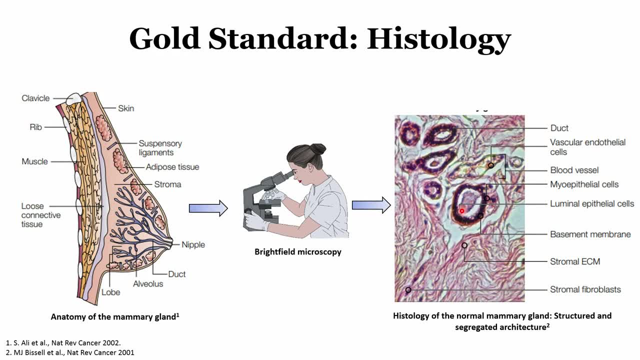 see the myoepithelial cells, luminal epithelial cells, that is, outer and inner structures of the basal membranes. and this is the complete basal membrane. over here you can see the extracellular matrix and then, finally, you can see the fibroblast which is surrounding or just lying around. 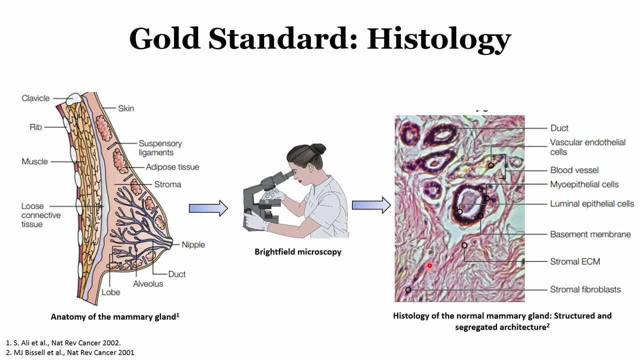 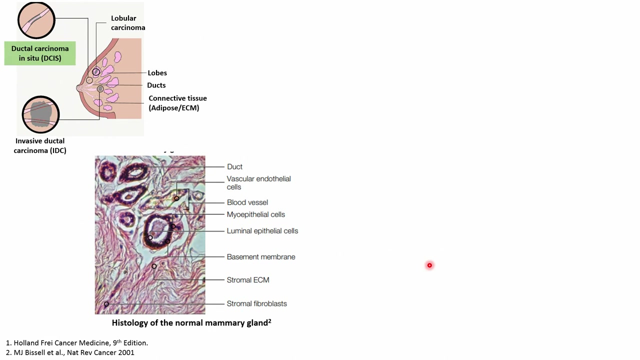 in the stroma. Now, what do we mean by ductal carcino in situ? is the cancer which is present, or the tumor which is present within the ducts, the gray part that you can see over here, inner surface of these ducts over here, which is not yet spreading to the outside the ducts. 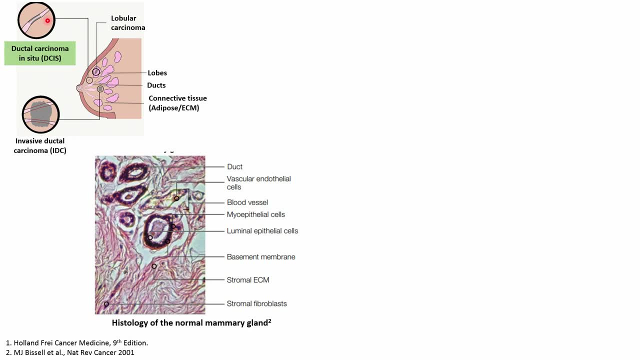 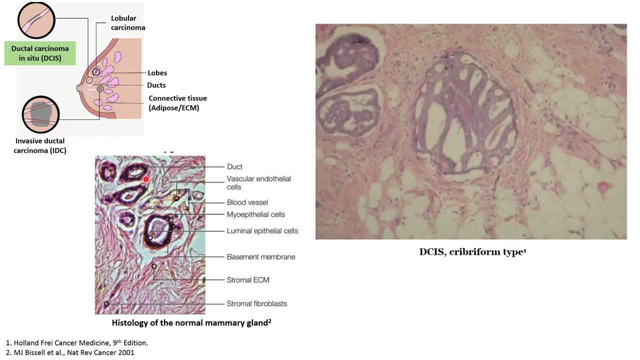 ok, That is the an important way to differentiate this with the other type of breast cancer. On the left side, again, we have the normal case, but on the right side now we have something new. So this is what you see is again. so we just give few seconds for you guys to think. 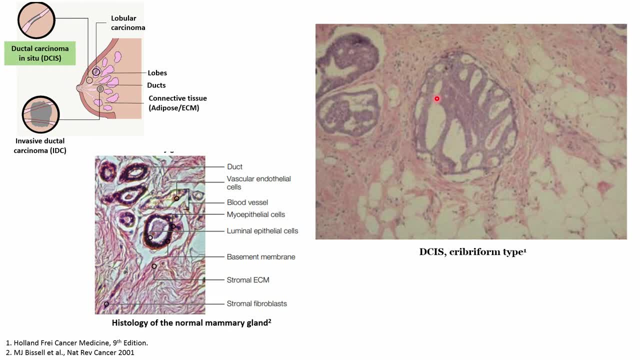 about this? what is this? yeah, So this is the ducts, ok, but this is a duct in the case of a diseased breast, ok, So what you see over here is the surrounding. over here is the- again, the basal membrane. 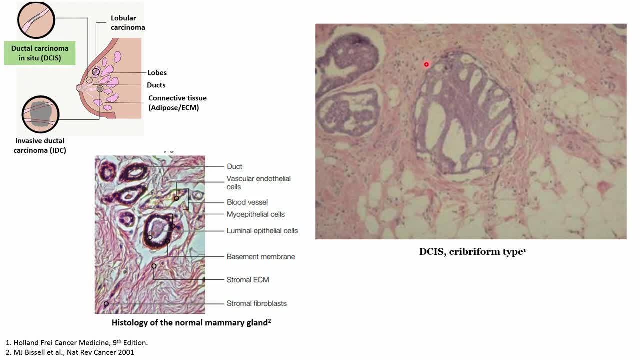 over here. but there is something else that you can see which is not seen in the actual case over here. that is the normal case of the ducts. So before proceed further, you can just pause this video and just think about it. what is? 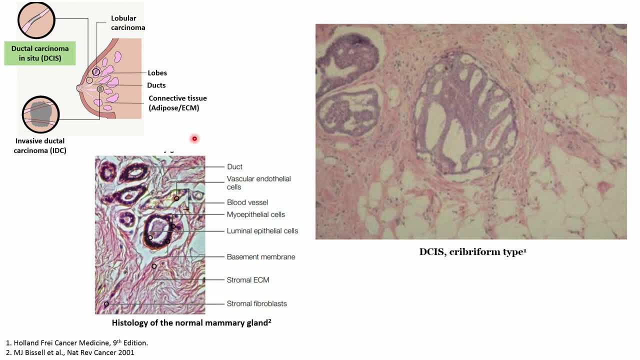 the difference that you see over here, as what that you cannot see in this ducts profile over here. So what you see over here that is different is the proliferation of the ductal cells. ok, So you earlier, in the case of normal ductal cells, you will see the hollow in the center. 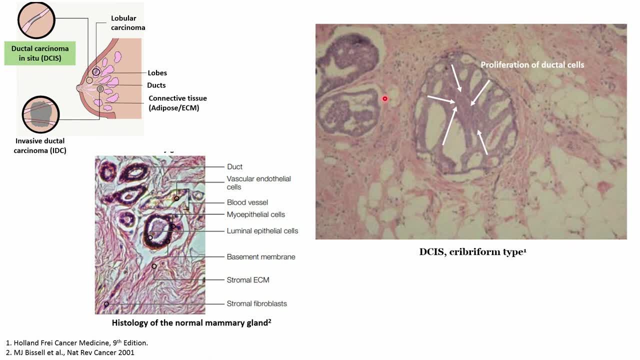 as you can see over here, but in this case, in the case of ductal carcinoma in situ, that is, the cancer which is inside the ducts as of now, which is not spreading outside the duct, is now proliferating inside the duct cell and it is obstructing the flow of milk. 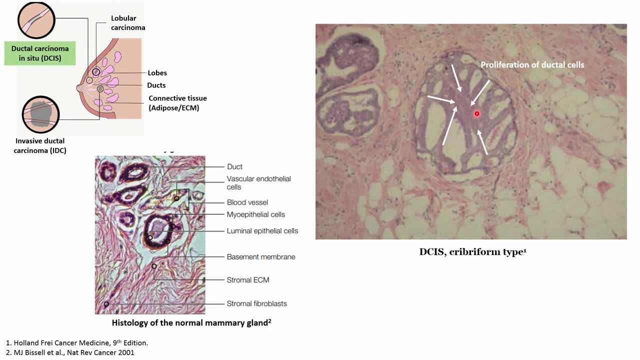 So what you see is having a new born with her right. So this type of the ductal carcinoma in situ is known as creed form type. ok, and there are different, even pathologies of the breast cancer that we will discuss, and one of them is creep. 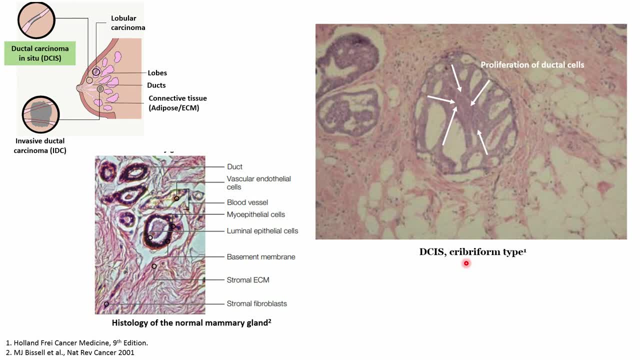 form type, but you can nicely see within the histopathological slides. Now as you go on and create your own devices, such as optical being one of this hypothesis to create such devices, it has the limitation to actually limit to diagnose the type of. 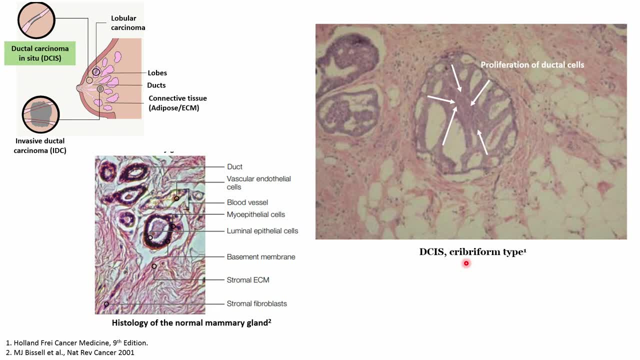 the tissues. So it becomes very, very challenging for the optical technology to actually also delineate or to specify which type of pathology of breast cancer is being present within the breast, And that is what you will see in the next few slides. so there are lot of different. 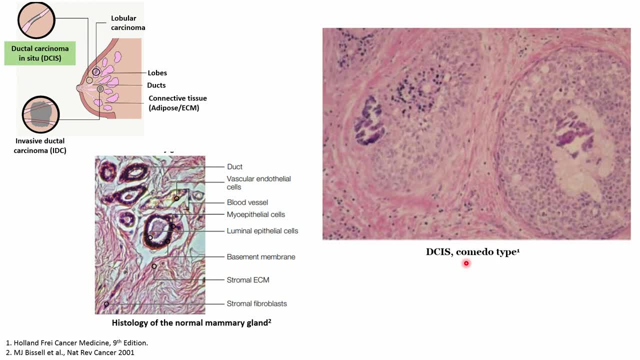 types of pathologies. So now, coming to the next type is the again its DCIS, that is, ductal carcinoma in situ. and now here you see something else, So you can pause the video for a few seconds and just try to see what are. what is the difference? 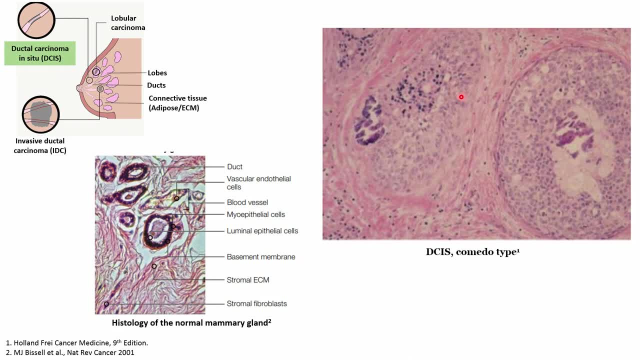 that you see in this staining image, which you cannot see in this original or the normal case of the ducts profile over here. yeah, So what you see is a fast again. this is the duct over here. ducts over here, ducts over here. 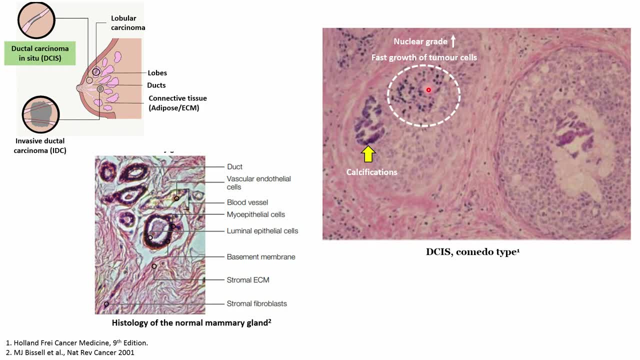 And what you see over here? because of the staining, it is actually in dark blue color. the dark blue color is the tumor cells and its growth is now very, very fast And that is why there is a large number of tumor cells within the ducts again, its surrounding. 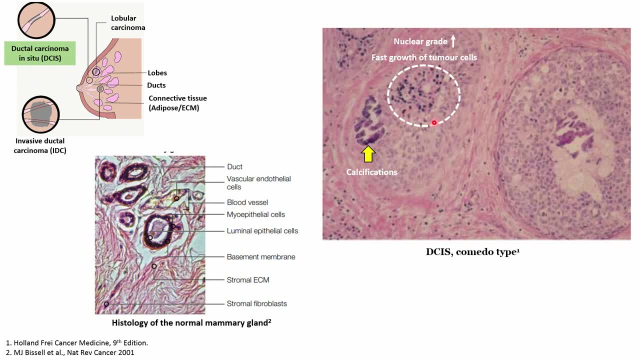 inside the ducts over here and it has a very high nuclear grade. that is, the growth rate of the tumor cells is very, very high, five high. In addition to it, what you see is the calcifications within now being formed within the ducts, and that is also a very important part, because calcification is also going to change the 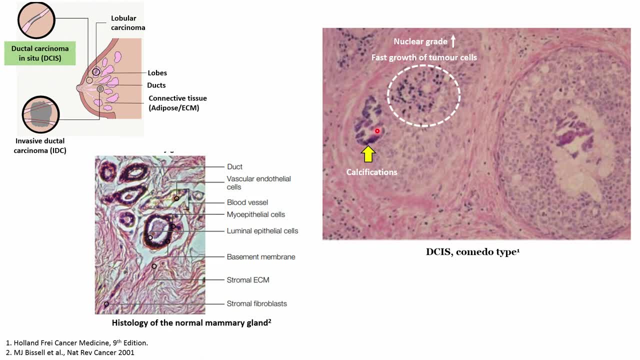 property, bulk property of the tissue, That is, the mechanical property of the tissue, eventually changing the optical properties of the tissue: 0, 5 00, 1. 1. again, it is still within the ducts. it is not yet spreading outside the ducts. So this: 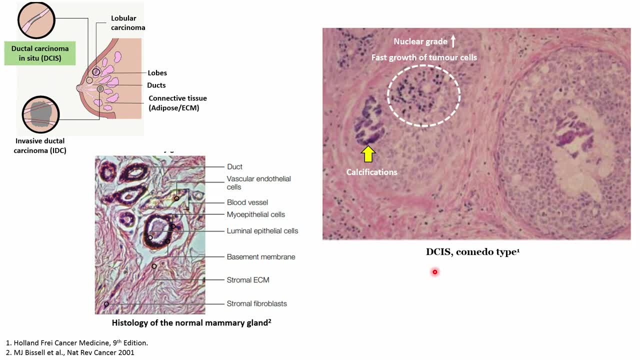 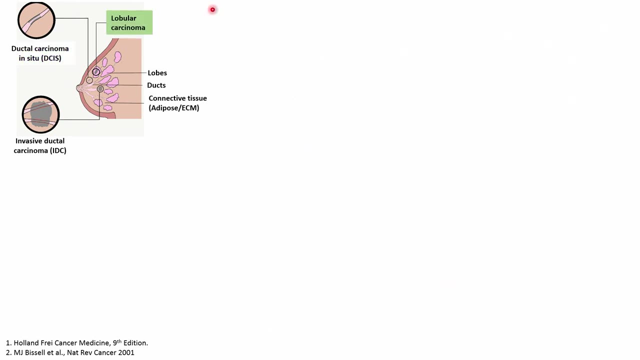 is a DCIS- ductal carcinoma in situ, and this type of pathology is known as comedotype. There are lot of other types of DCIS which you can go and refer to the other books, but we can go to the other part. that is now the lobular carcinoma. ok, That is present within. 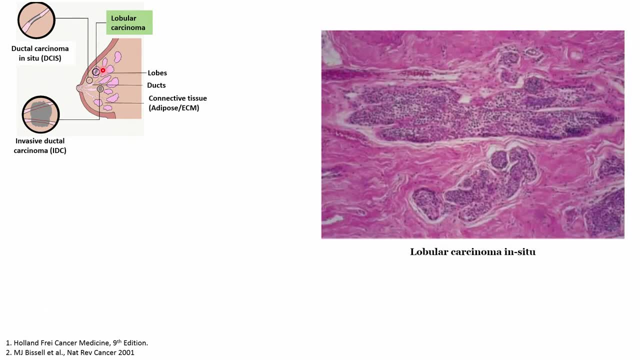 the lobes where the milk is being generated. So over here again, you can just take some time and see what is the difference over here that you can see as compared to the lobes over here. right, So you can see that it is. now the lobes is completely filled and dilated. 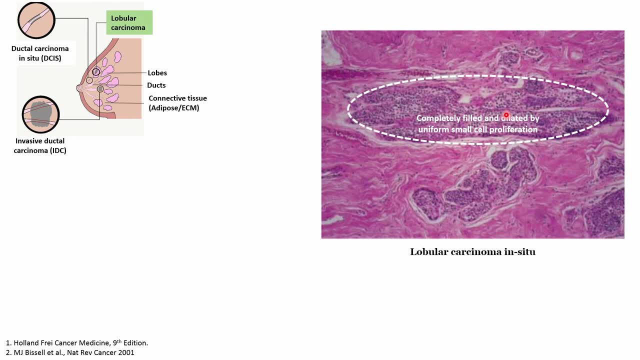 at which It is also important to know that it is being dilated, and it is dilated because, or dilated means it is now increasing it is own size and that is because it is getting completely filled, So it is no more space within this lobular cells or this lobular structure, and 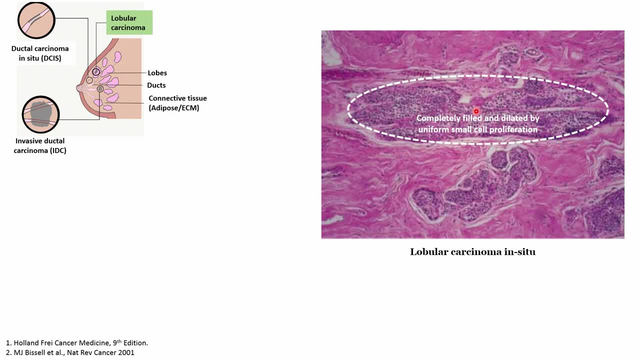 now it is trying to dilate or it is trying to increase its dimension, and that is because you are vielen cells over here, and now it is proliferated throughout the lobes. ok, But it is still not actually spreading out and that is why still in situ, ok, So we have. 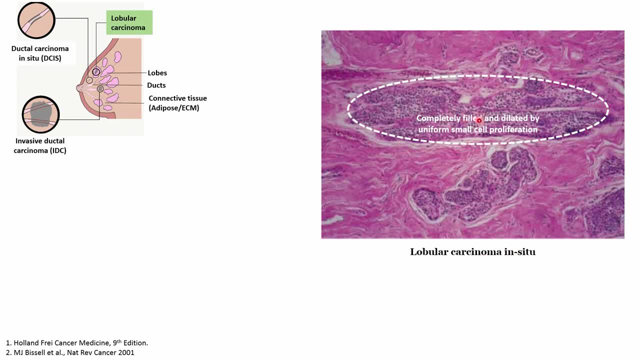 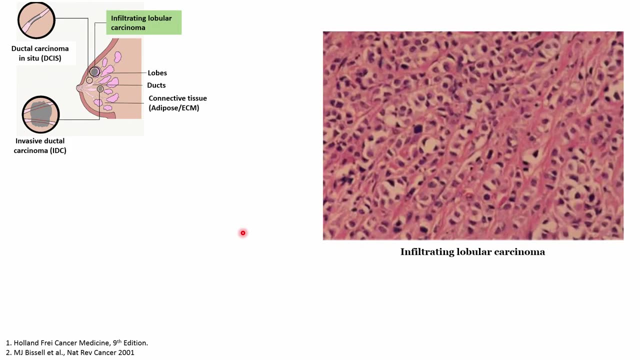 lobular carcinoma in situ. So it is still within the lobes and it is not spreading out of the lobes, vrai ہے? Ok, So let us go to the other part. We talked about in situ lobular carcinoma, but once 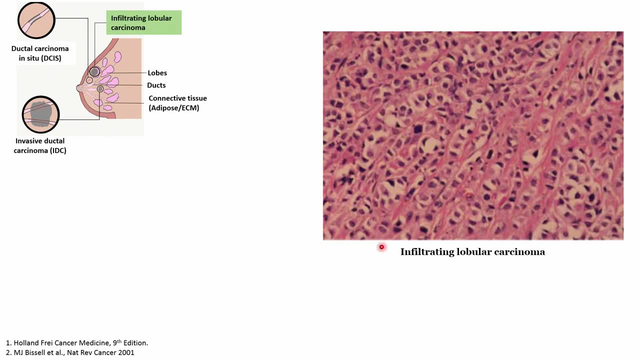 it starts to spread. what you see is something known as infiltrating. Infiltrating means it is now infiltrating to the other parts of the, of the of the breast, and then it will go to the lymph nodes and then it will start to put go to the other parts of the human. 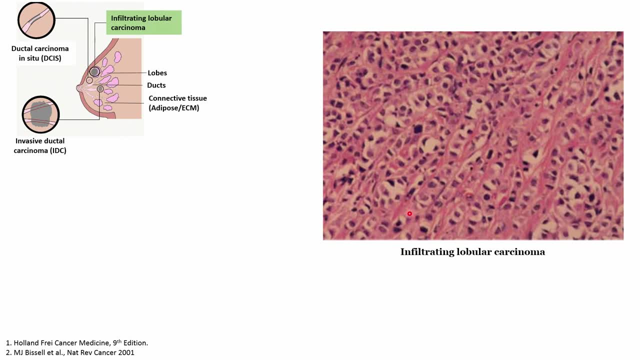 body. So what? how do you differentiate this with the other cells or the histopathology test that you saw? ok, So again, you can just pause the screen and just try to see. how do you? what is the type of the arrangement of the tumor cells that you see over here? 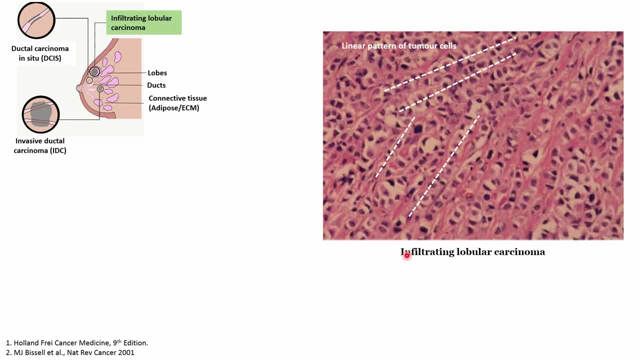 So what you see over here is a linear pattern of the tumor cells that you have not seen before. So this is a very obvious random arrangement of the tumor cells and very non-uniform arrangement. but in the case of infiltrating lobular carcinoma, what you see is a linear arrangement of the 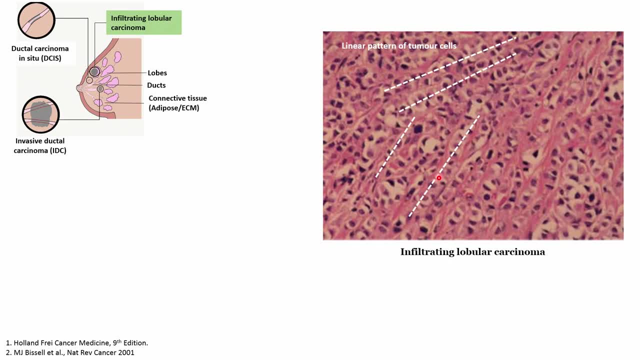 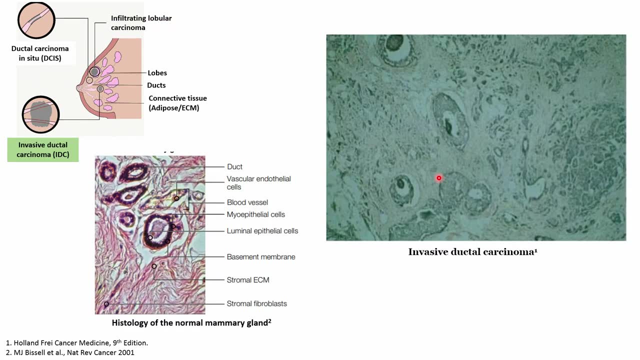 cancer cells. ok, So this is a way to differentiate this pathology with the other pathologies. Now let us, let us go to the other. that is the last one. This is the invasive ductal carcinoma. ok, and this is around 80 percent of the timesthat. 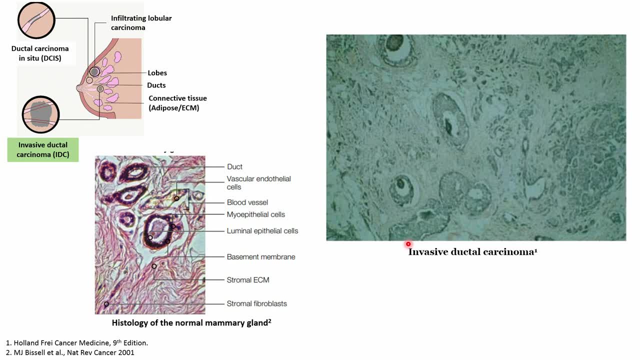 the clinician are able to see this kind ofor they are able to diagnose the breast cancer with the invasive ductal carcinoma and it is also famously knows as IDC, and it is a invasive ductal carcinoma. So, again, how do you differentiate it with the other pathologies? 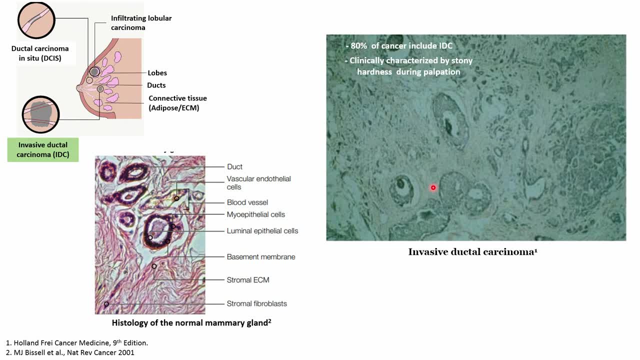 over here. it is actually clinically characterized by stony hardness during palpation. So palpation is a kind of procedure where the clinician tries to press the breast of the of the patient and try to see if there is some kind of a very hard structures like a lump structure. 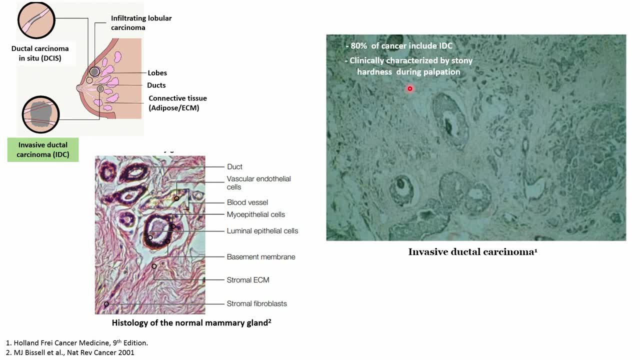 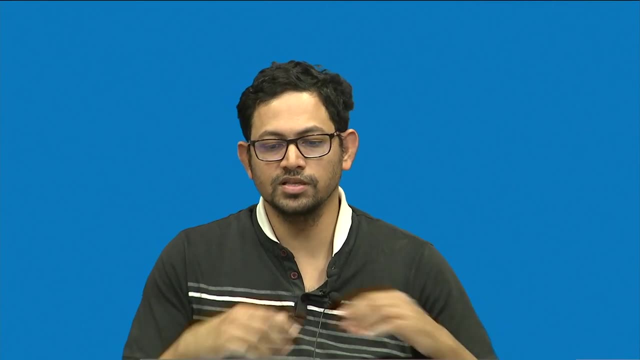 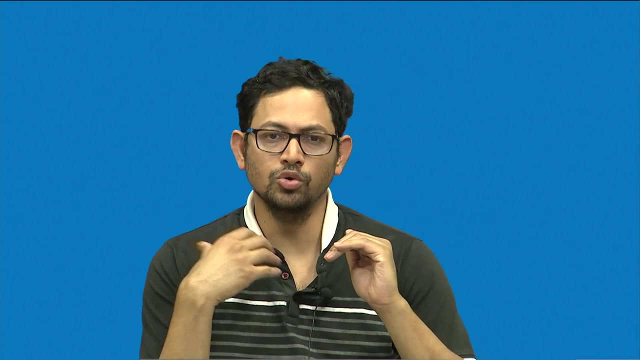 is present over here and it is very difficult to actually differentiate through the pathology over here. So let us go now forward to see the different types of techniques. different types of techniques other than histopathology, where we are trying to use the to diagnose the breast cancer. So, as you can see on the screen, there are 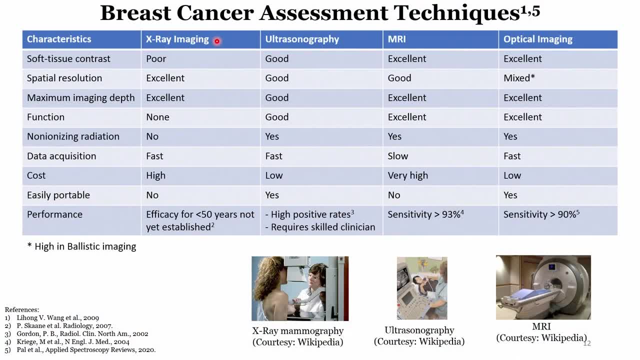 different techniques. the first one is the x-ray imaging, second is the ultrasonography and the third is the x-ray imaging. So the first one is the x-ray imaging, second is the x-ray imaging, third is the MRI, that is, magnetic resonance imaging, and then finally, 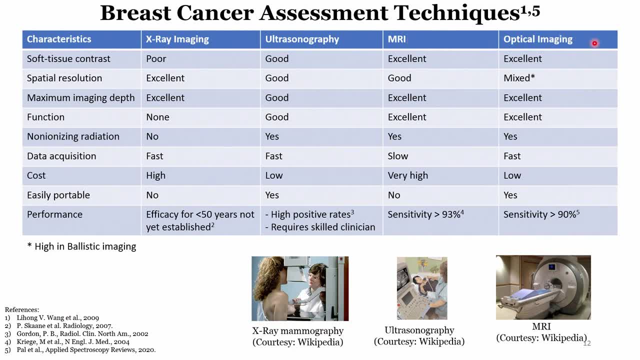 is the optical imaging. In today's course we will actually talk about the optical imaging. So there are different characteristics which are defined for these assessments. ok, For example, the soft tissue contrast. So in the case of soft tissue contrast, the ultrasound and MRI are like very, very good as compared to the x-ray imaging. 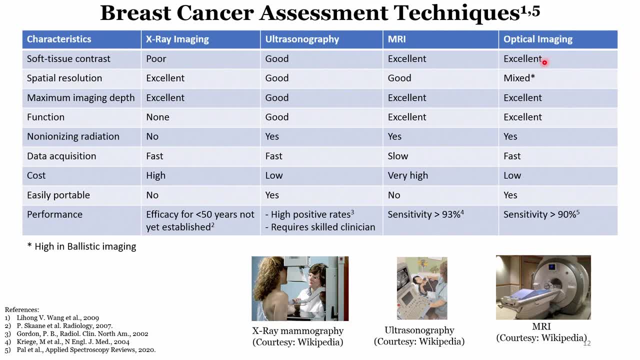 Even the optical imaging is very good in in the case of where you want to characterize soft tissue contrast, ok. So, for example, what does it mean? is you want to differentiate the tissue with the soft matters? ok, or the soft cartilage that is present? The next thing: 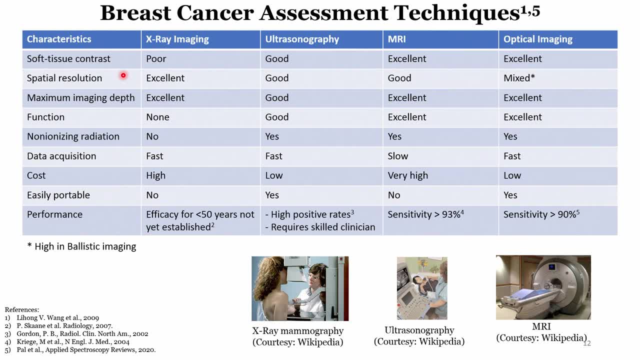 is the spatial resolution. So how nice resolution that you can actually get after doing the imaging. So in this case, the spatial resolution is excellent in the case of x-ray and it is good in the case of ultrasound and MRI, but in the case of optical it is mixed. So what? 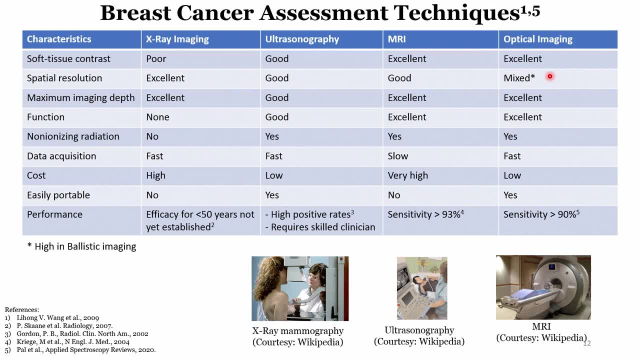 do we mean by mixed? is that, as you can understand, as you can, you will go. as you will see at a later stage, what you will observe is as the density of the breast is being increased, that is, the fat content is going to increase, So the density of the breast is going to. 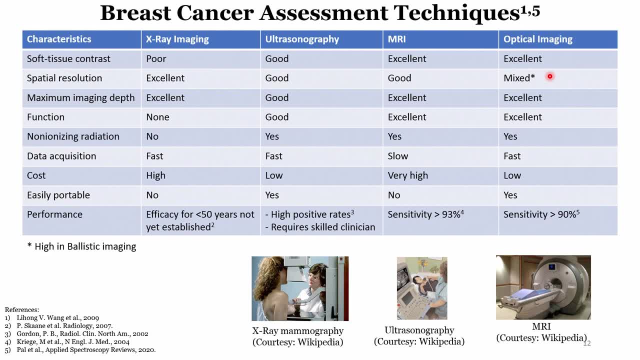 be more. in those cases, what you will see is that is more scattering, and as there is going to be more and more scattering, there is going to be loss of data. ok, So that is one of the major challenge: to actually diagnose the type of pathology that we were discussing. 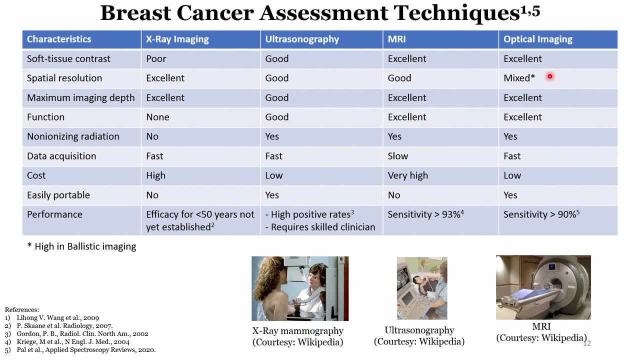 sometime back, ok, and low resolution is going to also affect our capability or our capacity to come to a informed decision. The next is the depth of imaging. in the case of x-ray, which is a ionizing media or ionizing approach, is excellent because it is able to pass through the tissues very nicely In the 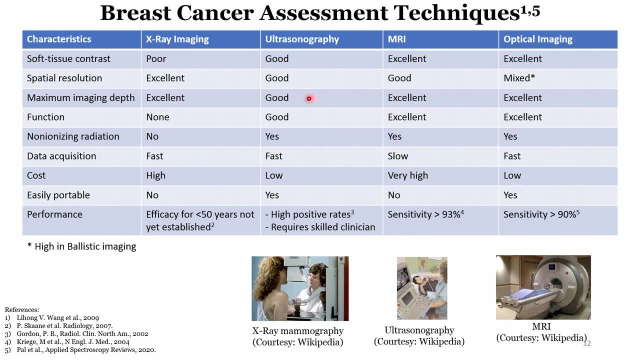 case of ultrasound it is good, and in the case of MRI, again, it is a kind of an x-ray. So it is of course excellent. In the kind of case of optical it is depends on the operating wavelength. So as you go on increasing the wavelength, in order of mid, 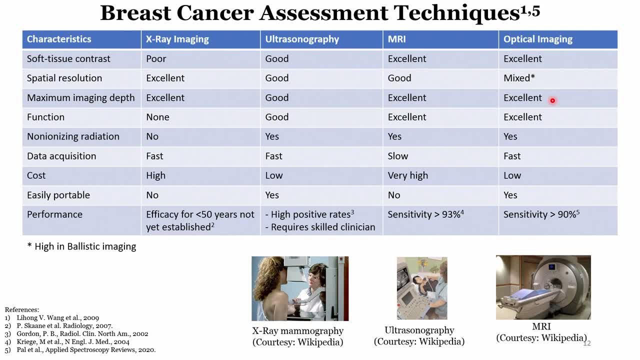 infrared regions or near infrared regions, you go ahead with penetrating large distance through the breast tissues At the lower wavelength, such as the visible wavelengths. in such wavelengths there is lot of scattering, So it depends on which wavelength are using for over here, in the case of optical, The functioning. so you want to also know. 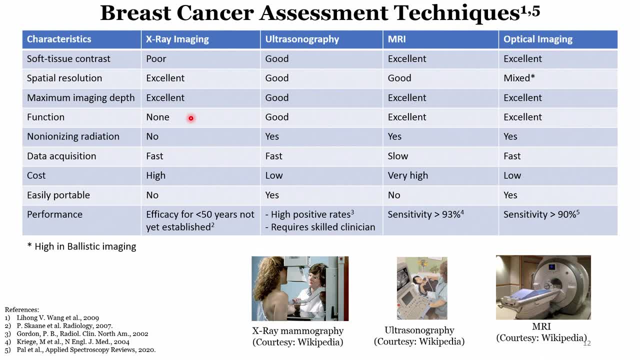 the type of analysis that your breast is performing. For example, you want to know oxygen saturation. So that is with respect to some work I am doing. For example, I am doing a muscular twitching of my hands, I am quenching my fist. In such cases, what you will see is that my 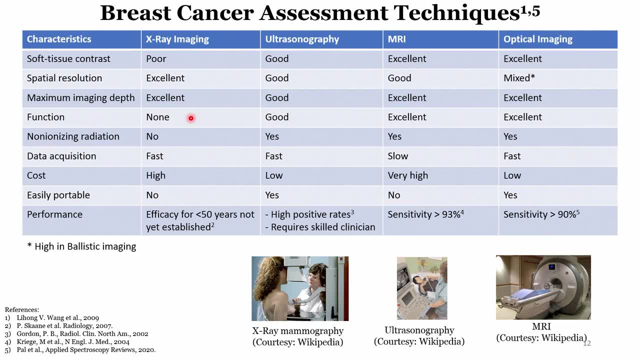 brain, for example, will work in a different way when I am doing a certain kind of function. So functional MRI is the something new that has become and that is also excellent to understand how good we are doing that particular function. So in x-ray imaging that is not possible. 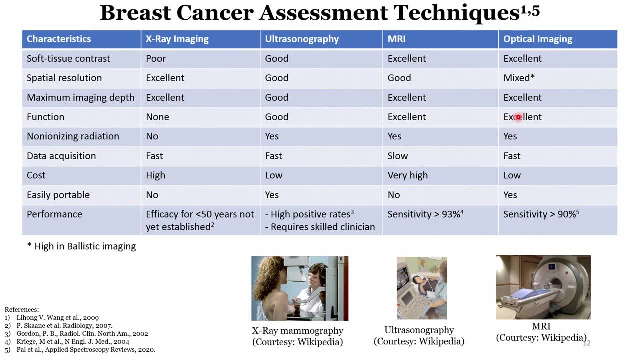 In ultrasonography it is still possible and it excellent in the case of optical imaging. Let us see now which one is non-ionizing. Of course x-ray is non-ionizing and ultrasonography is still higher. So actually x-ray is actually ionizing and the rest of them is non-ionizing. 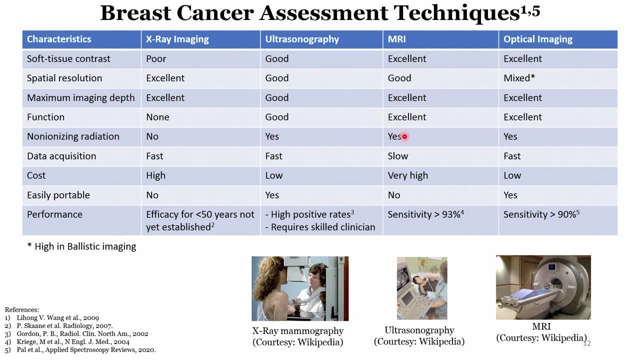 In the case of magnetic resonance imaging we are using these electromagnetic fields with the coil structures and with the particular frequencies over here. So if you talk about the computer aided automation, that is the CAT scan, computer aided technology, So in such kind of CAT scan it is still actually x-ray imaging. 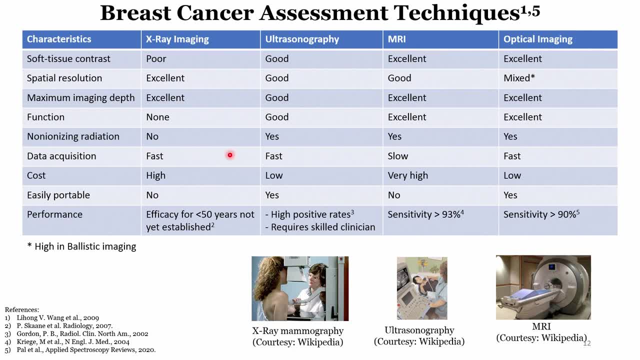 Data acquisition is actually very fast in the case of x-ray imaging, ultrasonography and optical imaging, but in the case of MRI it is comparatively or relatively slow. Cost is very high. for x-ray mammography the dimension is also very high, so the it reduces. 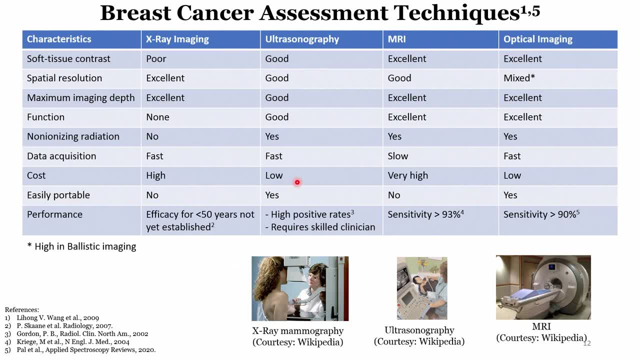 the portability. In the case of ultrasonography, The cost is low and still portable. In MRI it is cost is very, very high and it is not portable because the dimension, as you can see on the right side, is like huge. For the cost of the optical imaging is low because we use technologies such as lasers. 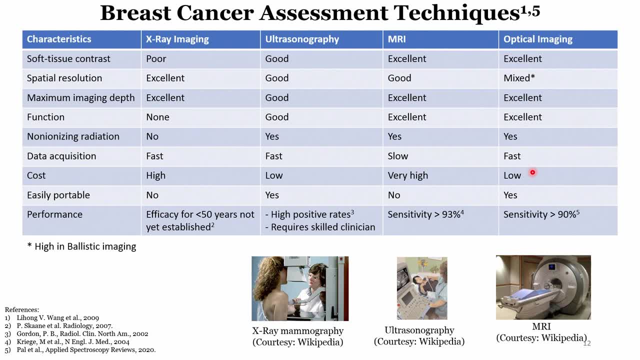 as well as LEDs And such techniques could be actually used. They should be used to differentiate or to quantify the bulk optical property like scattering coefficient and absorption coefficient. so the cost of the LEDs and lasers are comparatively lower and the diamond sense of such sources. 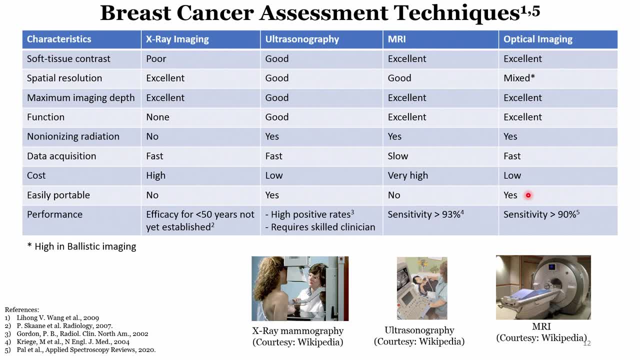 are also very lower, So it becomes portable. So you use lasers and LED as a source and detectors. you use infra detectors, for example, or you can use the ph bracelets. Yes, use the photon silicon detectors. you can use photomultiplier tubes. all of them are. 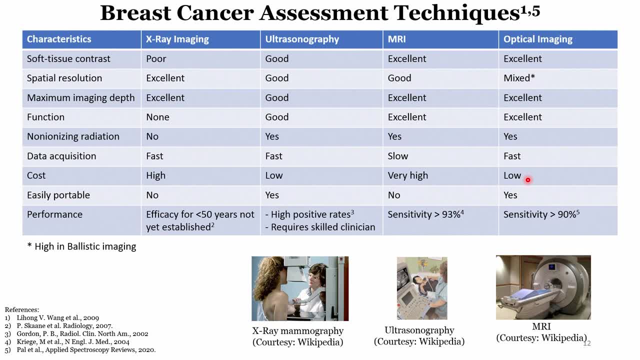 kind of a detectors. Again, those detectors are small in dimension and it is actually because it is small you can actually make it a very portable device. Performance wise, efficacy means the concern with the X-ray mammography is that the efficacy for people or women less than 50 years is not yet established, because it is not advisable.